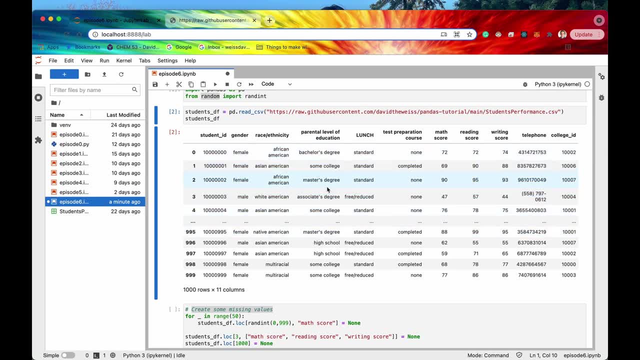 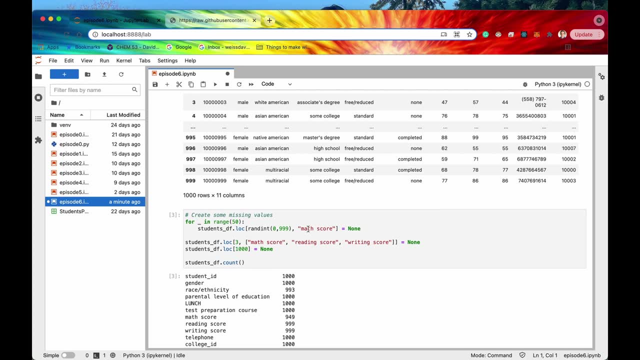 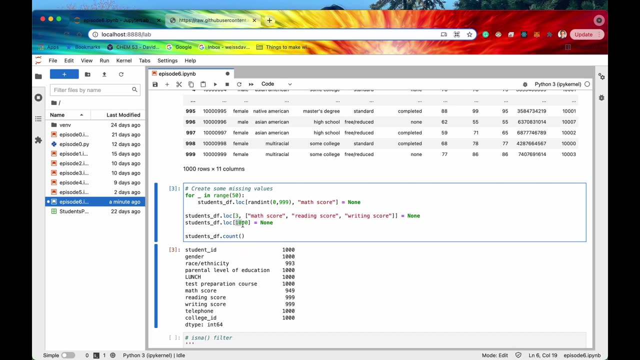 real world scenario. you'll most likely have missing values within your data frame, So all this cell is doing is just emulating that. We're just going to be randomly creating some missing values in the math score column, as well as these columns in record three, And also we're going to 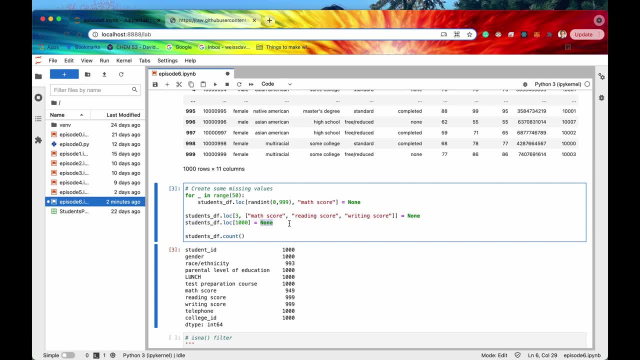 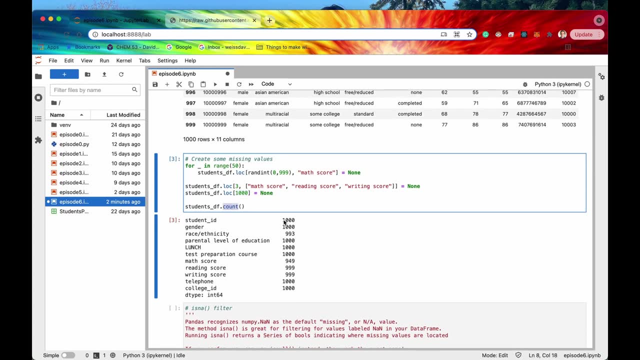 create an entire row that has missing values for every single column And that's going to be labeled as record 1,000.. Awesome, So now let's count up all of the non-null values in each of these columns So it looks like again we have some missing values in the race: ethnicity. 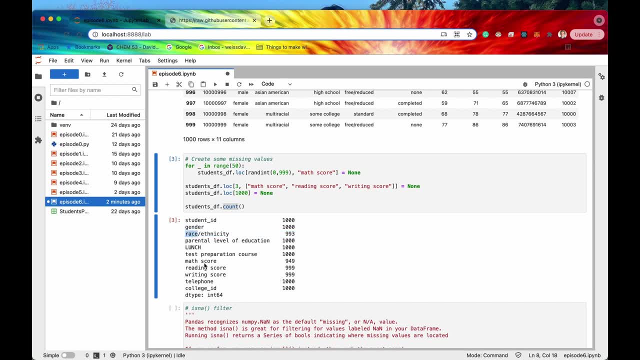 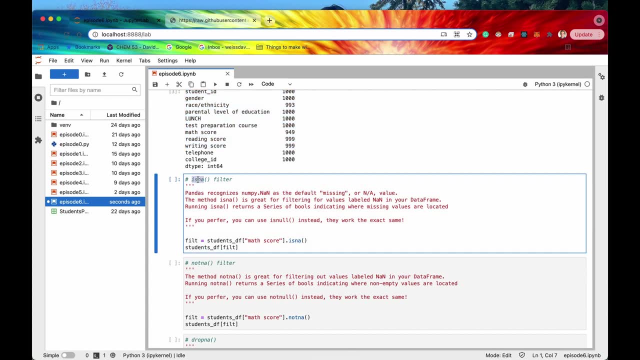 or missing values in the race, ethnicity column, math score column, reading and writing score columns. All right, So let's take a look at our first method. So this method is NA. Basically, it's going to tell us where in our data. 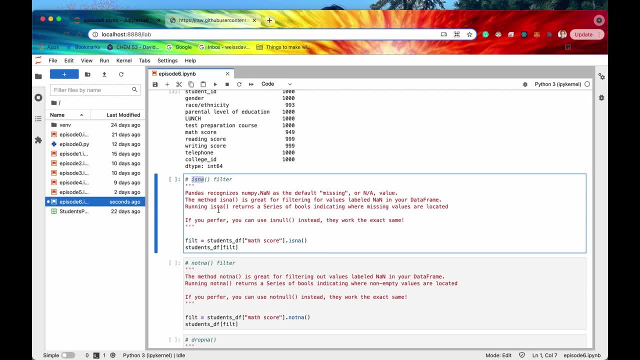 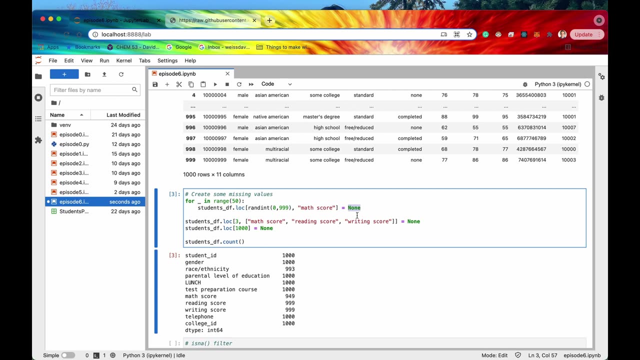 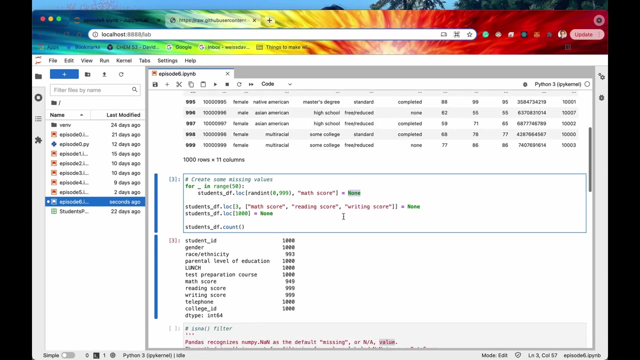 frame is our missing values. So, just as a word for information, it's important to note that pandas recognizes numpynan as the default missing value. So, if you recall, when we assigned missing values, we assigned it to the Python: none data type right. However, when we did that, pandas 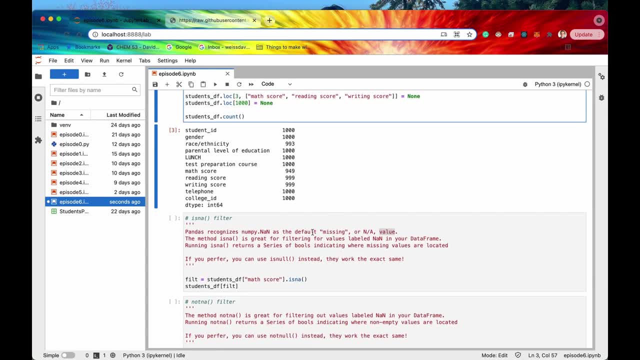 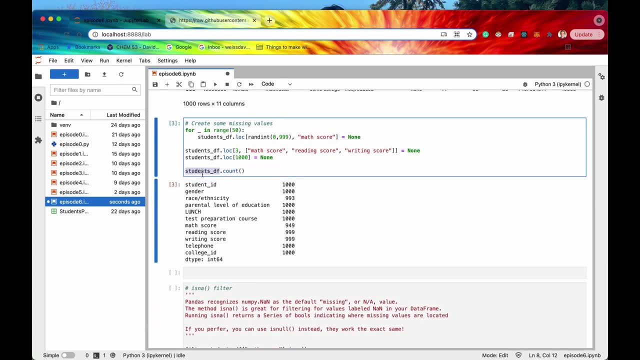 automatically converted none to its default missing value. So we're going to take a look at the default missing value, which is numpynan. So let's take actually a quick look at that before we proceed. I'm just going to quickly show that in this cell. So here we go Again. look this. 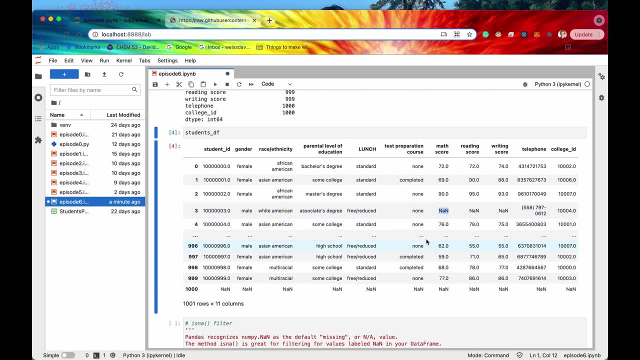 value in record three is nan. That is pandas way of saying that this is missing. This value is missing Also. look at this. This is pretty hilarious. Right here we have an entire row full of missing values which are nan's Awesome. Let me now delete that. 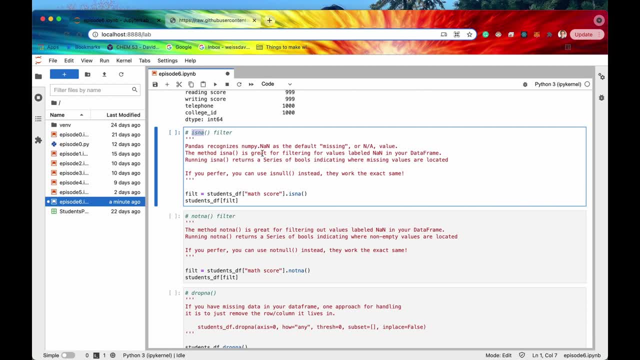 Cool. So again, is na is great for filtering for values labeled nan in your data frame. Again, these are the missing values, Because is na returns a series of booleans indicating where missing values are located And, if you recall from our filtering episode, whenever we have a series. 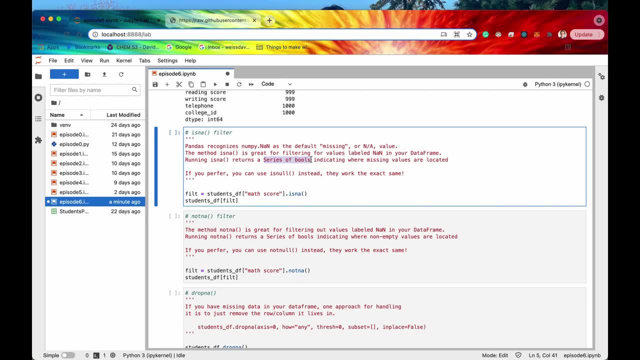 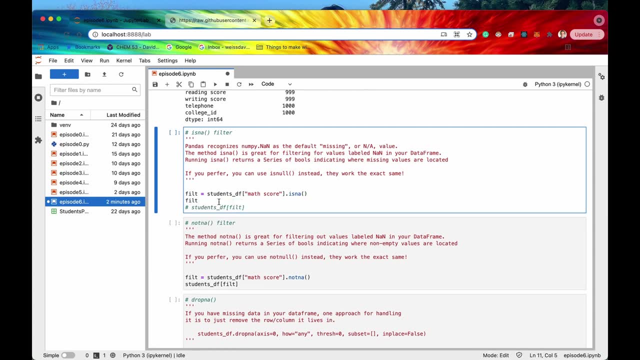 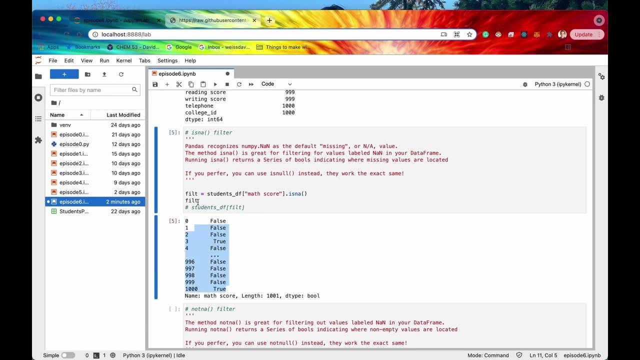 of boolean values. that means that we can use that as a filter mask. So let me just quickly show you that You haven't seen that episode on filtering yet, which I would recommend that you do. All right, So here we go. We have our series of booleans. Now we're going to use that filter. 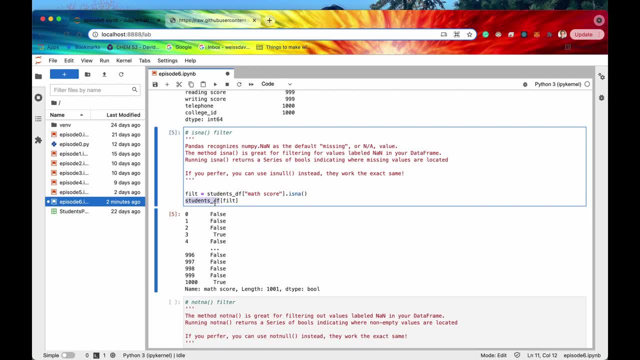 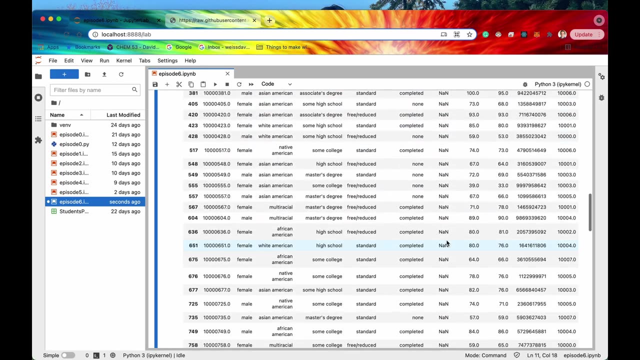 mask that series to filter for all of the values in the math score column that has or that is missing. If I run this cell, here we go: Math score. here's the column right here, As we can see as we scroll down, all of these values are missing because they are not missing. So we're. 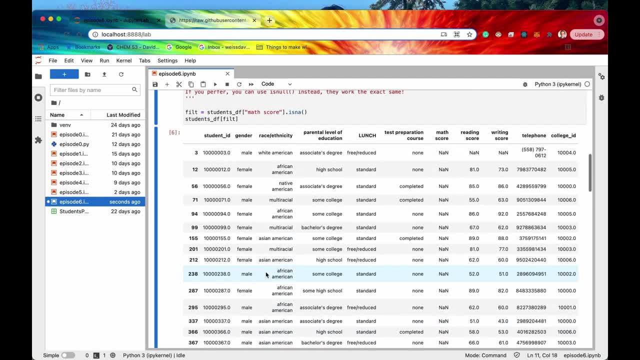 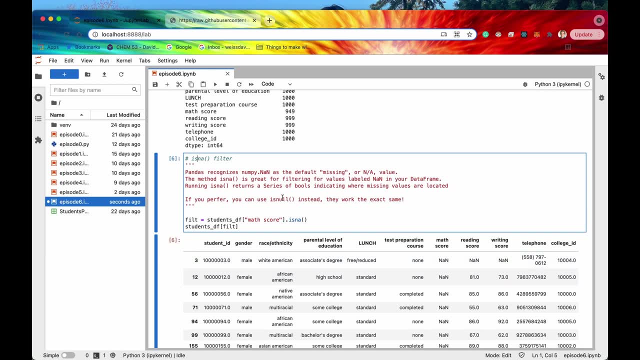 so now we have all of the records right of this data frame where we have missing values for math score. Cool. So one more thing before we proceed to the next method we can also use: is null for this exact same operation. Is null is just an alias for is na. These two methods work, the exact. 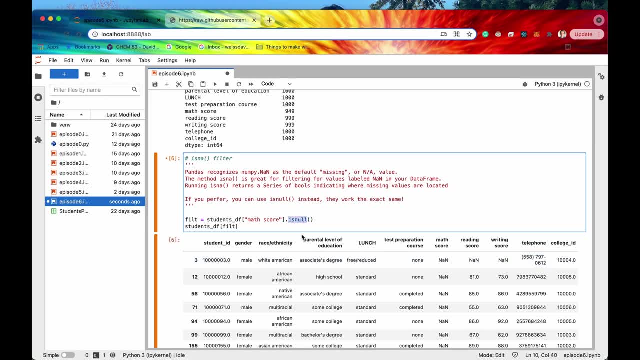 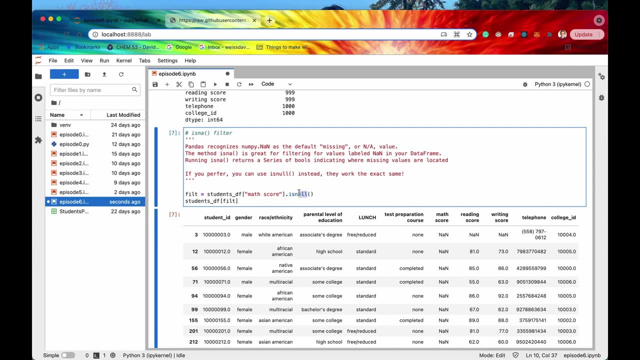 same way. In fact, I believe that is null, just calls is na, So they have basically the same performance. Whichever one you want to use, that's totally fine. It's just personalization, Personal preference, As we can see again. yep, this, this returns the same, the same data frame. 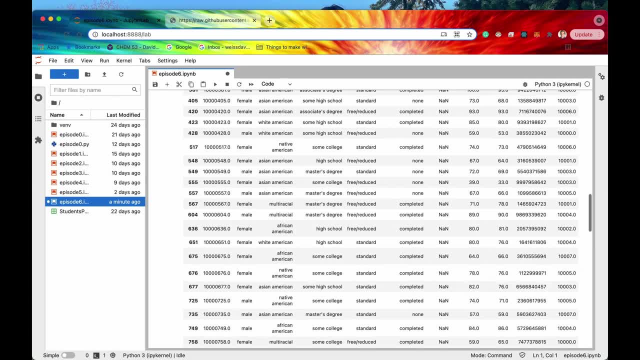 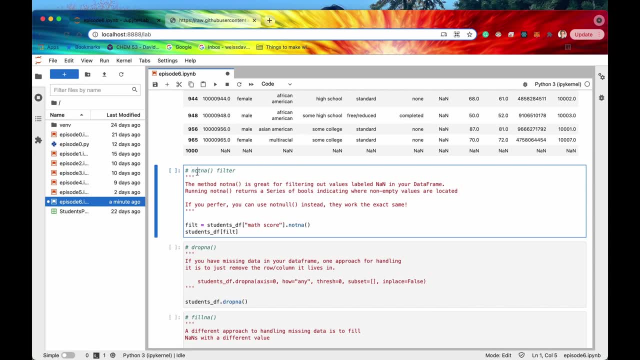 as is na Cool. Now let's move on to the next method. The next method works basically the same exact way, but it just gets the opposite rows right, So not na is going to return us that same series of booleans. However, instead of indicating where there are missing values, 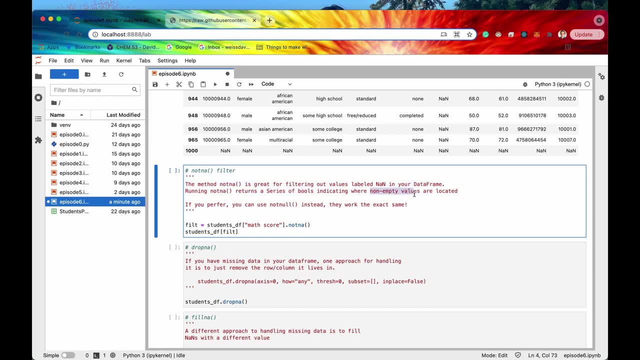 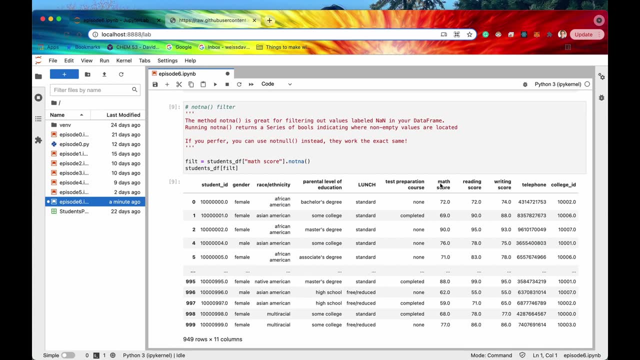 where there are na n's. it's going to indicate where there are not missing values. So again, it works the exact same way. However, it's going to get us all of the rows in our math score column that have real values, not missing values, in our math score column- Awesome, So this also. 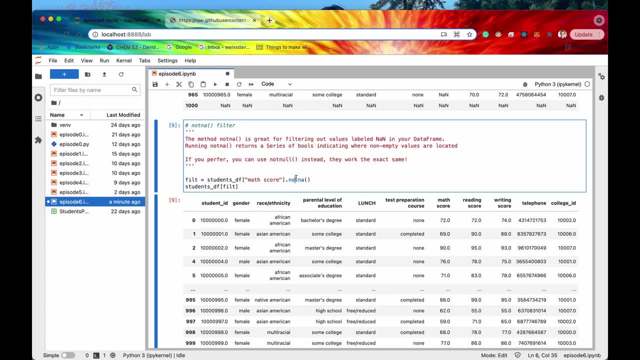 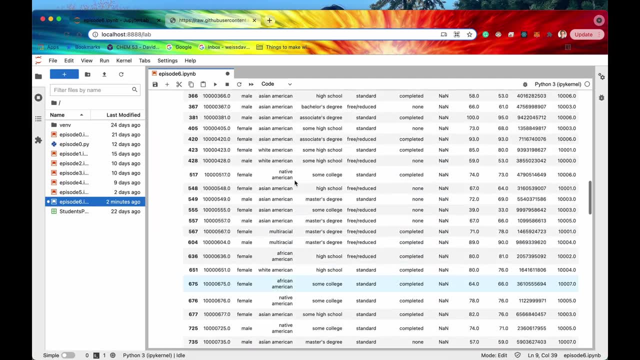 has the- not null- method. Again, whichever one you want to define, that is perfectly fine. But I do want to mention one more thing, and that is: this method, not na, performs the same exact way as if you're using the same exact method, but you're using the same exact method, but you're using the. 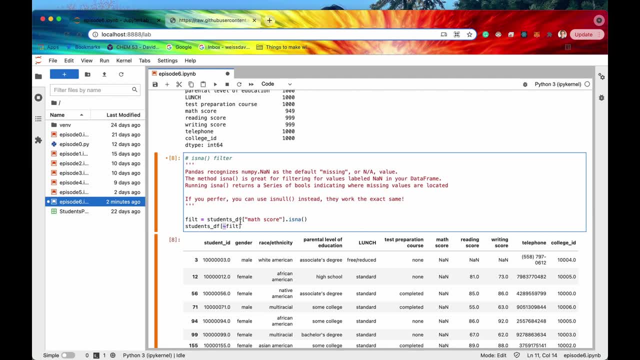 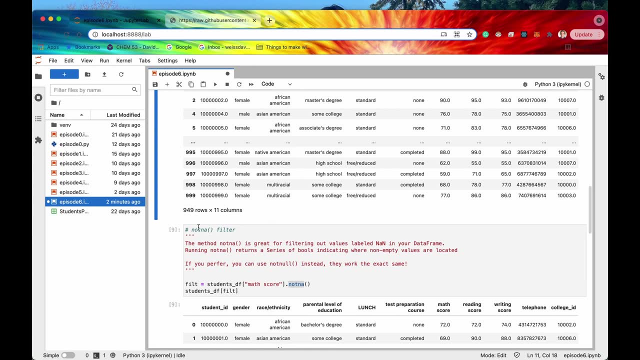 same exact way as if you're using the same exact method. but you're using the same exact method, but you're just to give this filter the not operator right. So again, this works the exact same way, saying not filter as just using not na right. So not is na is the same thing as not na, It's just. 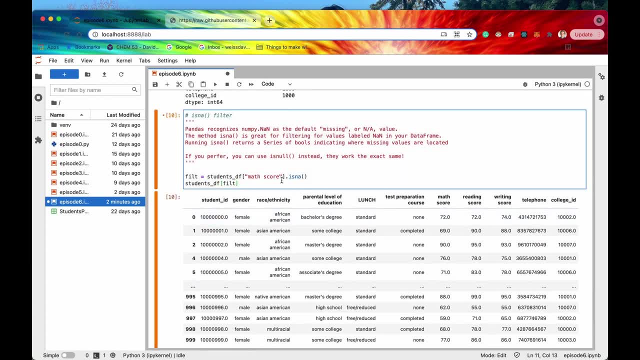 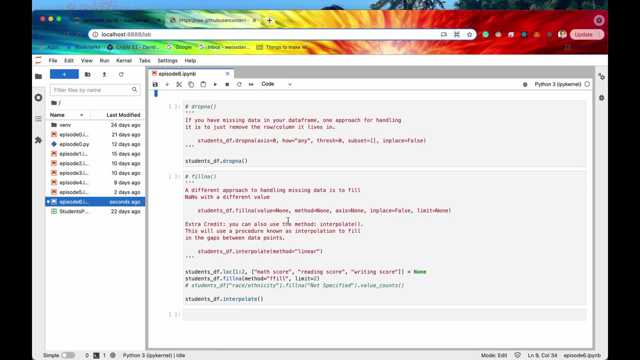 whatever you want to, however you want to do it, I personally like not na, just because it's a little bit more legible and human readable. All right, let's move on to our next two methods, which are: drop na and fill na. So now that we've done that, let's move on to our next two methods, which are: 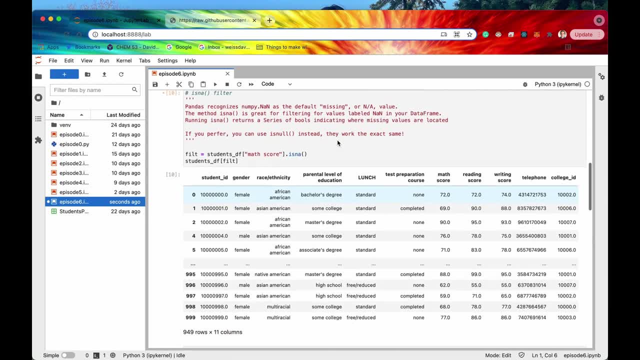 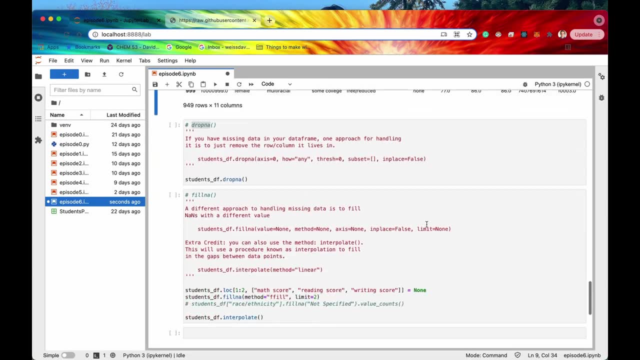 drop na and fill na. So now that we've done that, let's move on to our next two methods, which are know where our na values or our na records are. what are we going to do about that? So there are two different ways which we could handle those na values. We could just literally delete the entire. 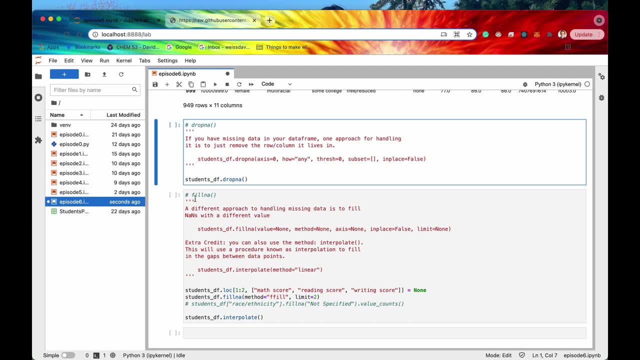 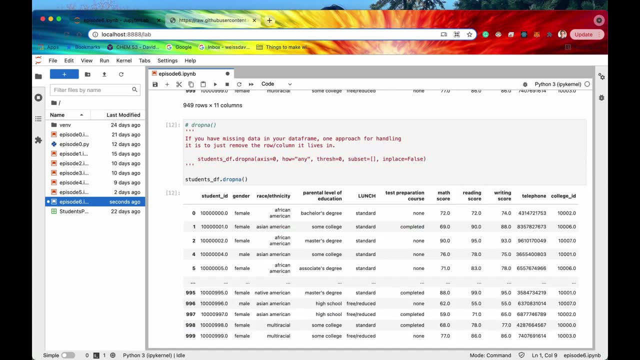 record that has that na, or we could fill that missing value with another value, So let's first look at dropping the value. All right, cool. So if I were to run this cell right here, what that's going to do is it's going to look through the entire data frame and it's going to look through. 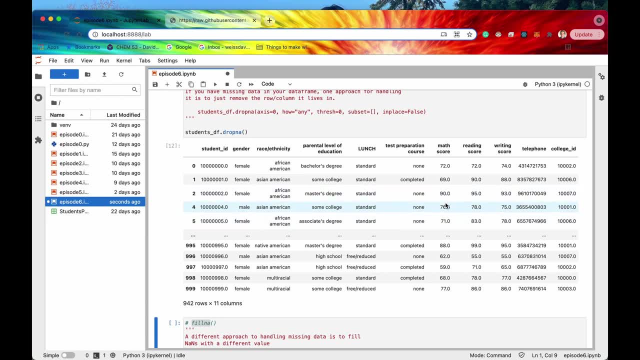 the entire data frame. If there is a missing value, which again is a na? n value, then it's going to drop in any like in any of the cells, then it's going to drop that entire record. Now let's say that we didn't want to drop the entire record. we want to drop the entire column of that, wherever. 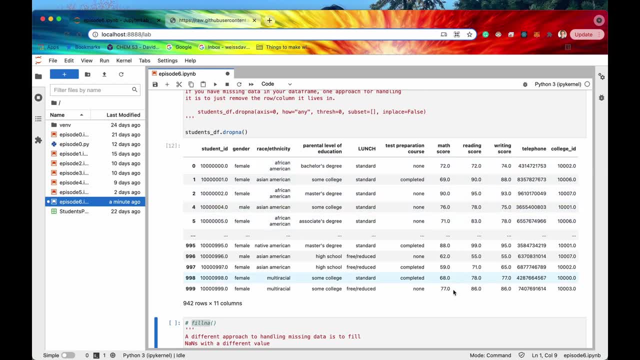 there is like an na n. instead of dropping the record, we drop the column. Well, we can just specify that when we say axis equals one, again one indicates that it is a column. However, if we run the cell right now, it's actually going to not return anything, Because, if you recall this, 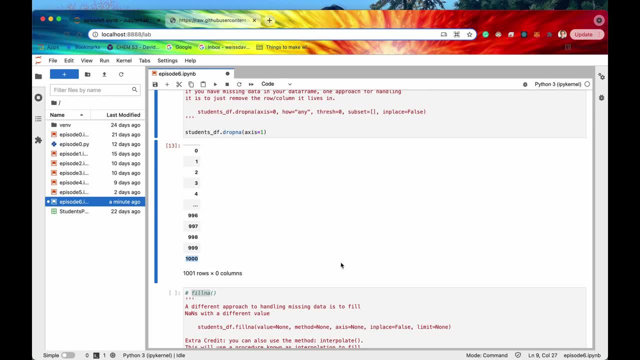 last record with index 1000 has an na for every single value. So what this is doing is basically just dropping every single column because every single value in this record is na Awesome. Let's just take a quick look at some of these other optional arguments. I'm not going to go through. 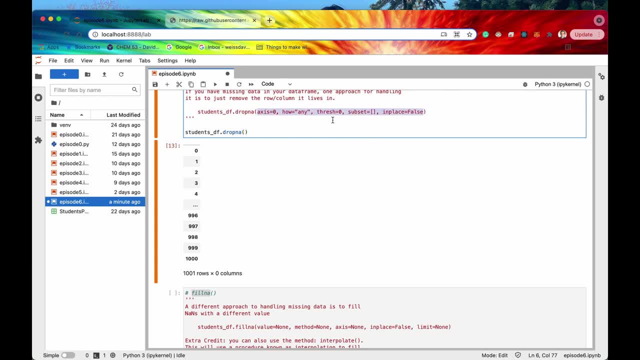 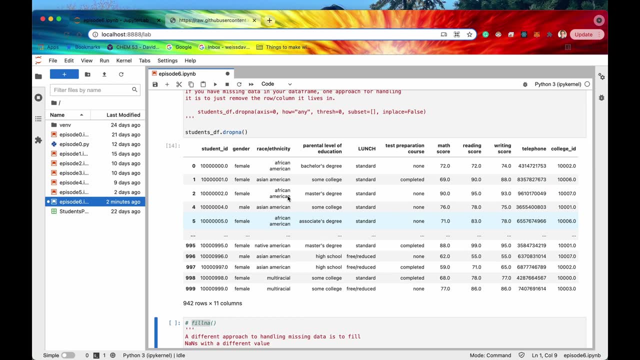 all of them, because I think you can do that in your own practicing. But let's look at subset. So if I were to say drop na. however, I only want to look at, say, the math score column, then I could do that right. I could say: subset is equal to, and now I'm going to say: math score Awesome. 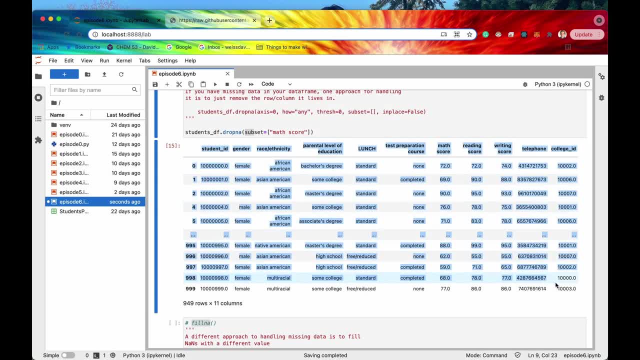 What. so what this is doing is, instead of looking through the entire data frame for na n values, it's only going to look at the math score column, And if there is a na n value in the math score column, I'm going to delete the entire record. However, I don't have to look at math score. let's say I want. 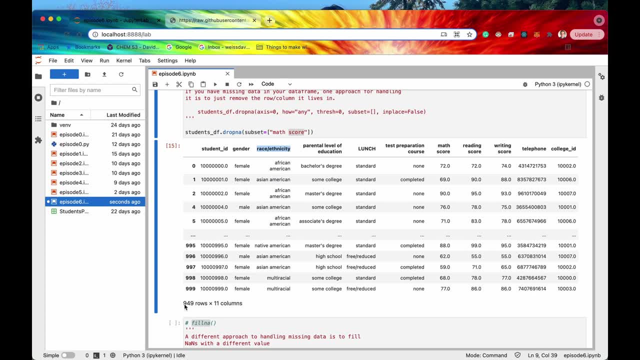 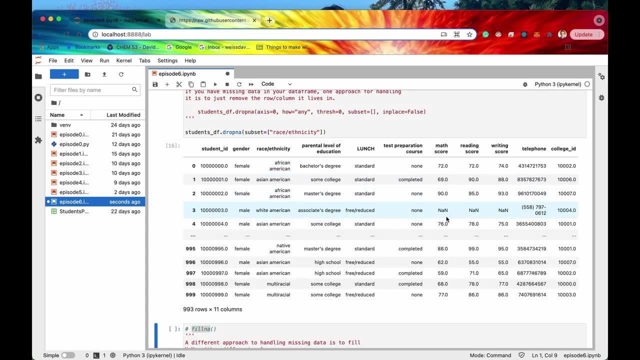 to look at race or ethnicity. So again, look, there's 949 rows. But if instead I supply this optional argument with race ethnicity, then now this column right here, record three, or I mean this row, did not get dropped, because there is indeed a genuine value in race ethnicity, right. 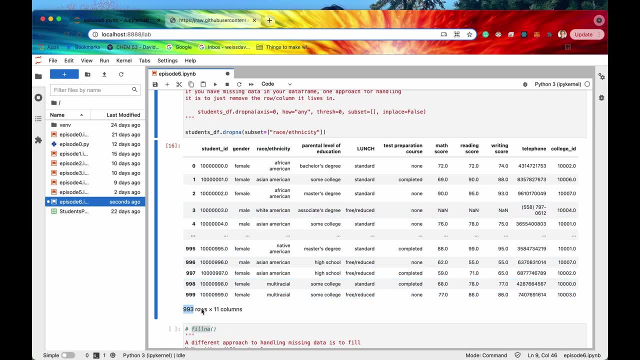 here I dropped a couple rows, But again this row was not dropped, even though there are na n values, because there was a genuine value right here in the race ethnicity column- Awesome. So let's look at how. just just because if we were to say how, right now the default is any. but if I were to 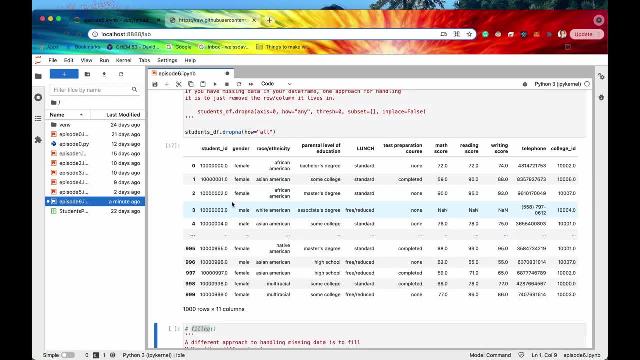 specify how equals all. what that's going to do is it's actually going to look for na n values right throughout the entire data frame. So if I were to say, Thresh this method, I mean this optional argument, could be somewhat complicated to learn at. 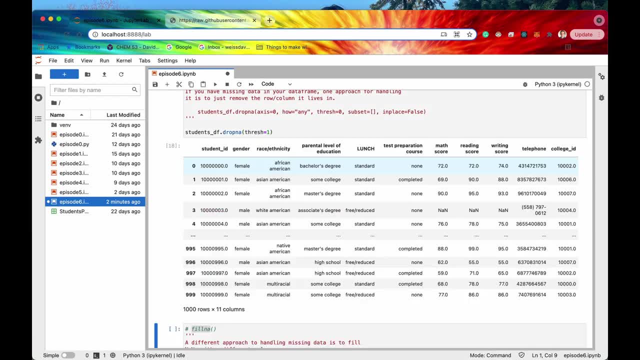 first, but let's say: Thresh equals one. what this is doing is that? what we're specifying is that before you drop the column- like let's say that you find, let's say that pandas finds a missing value, Before we drop the entire row. 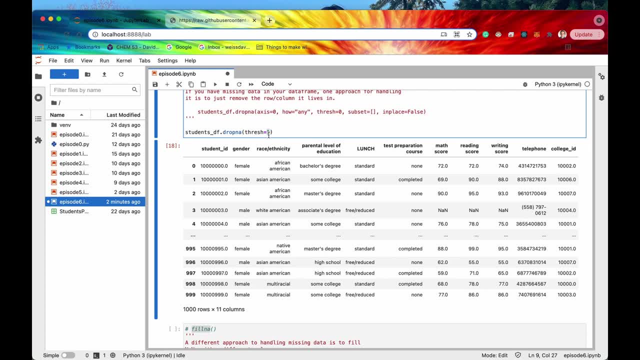 First, let's check to see if there is at least one value in that row that is genuine. So, for instance, this third record, this third record, right here it found an na? n value, but we saw there was at least one value that was real. 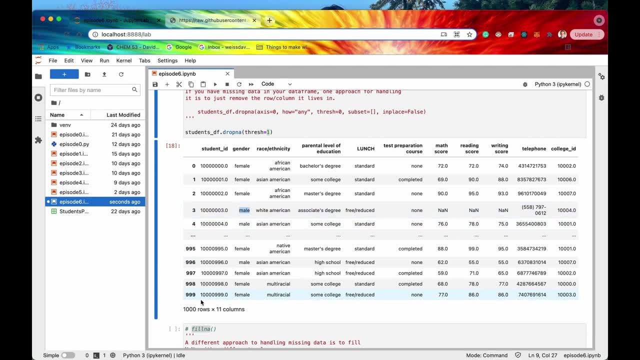 So we decided not to drop that record. The last row definitely did get dropped because there are no values in this row that are real, But let's take again a look at this row three. So we got one, two, three, four, five, six, seven, eight different values in this row which are real. 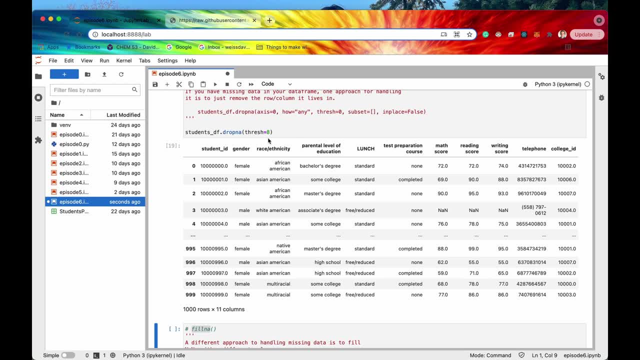 Right. So if I were to say Thresh equals eight, Yup, Looks like this record still exists. But if I were to say now, Thresh equals eight, Yep, looks like this record still exists. But if I were to say now, Thresh equals eight. 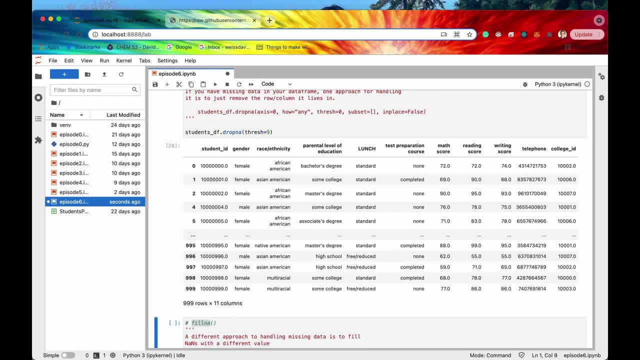 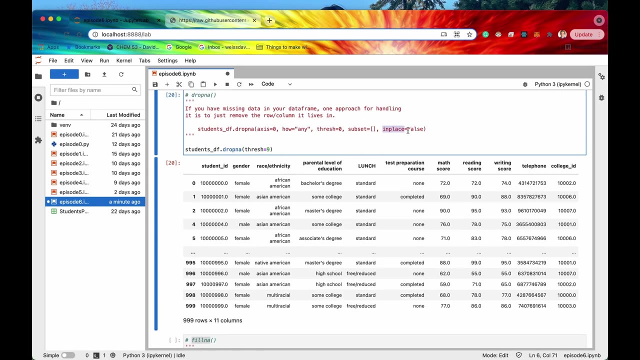 So if I were to say now, Thresh equals eight, equals nine, which is a pretty high threshold, but if i were to say that then look, now this record got dropped because there wasn't at least nine values that were not missing in that record. awesome, so in place, let's. just because this is the last optional argument, let's just go over it. 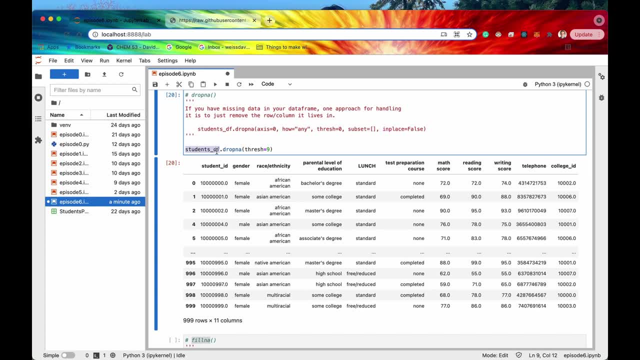 so in place. what that does is that, instead of like making a copy of students data frame- that's what we're doing right now- we're making a copy of it and then producing that as the output. if you specify in place equals true, what that's going to do is directly affect this data frame. uh, the, the. 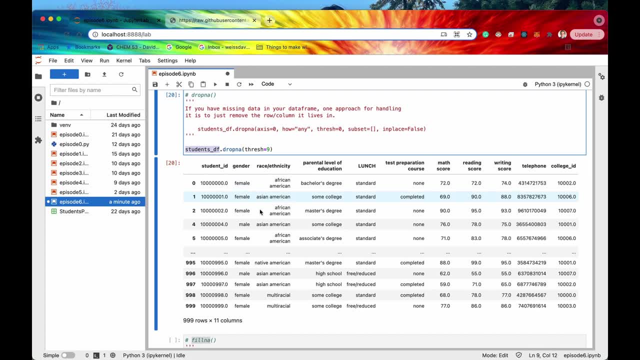 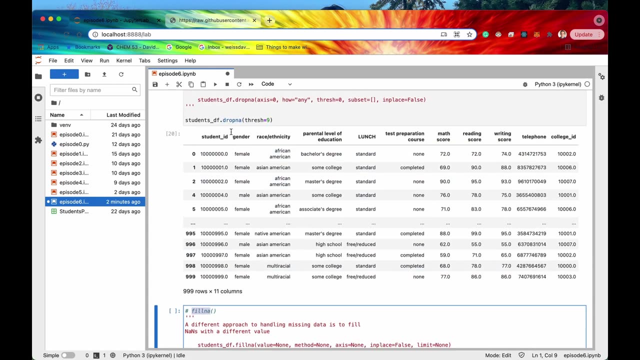 actual data stored under this variable name: students, data frame. cool, so i would recommend, on your own time, try that out and see what that does. awesome, so let's move on to the next method, then, which is fill na. so, instead of just dropping the entire row or column, what we can do if we find 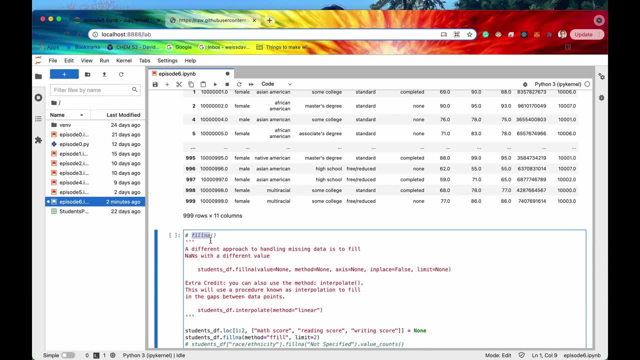 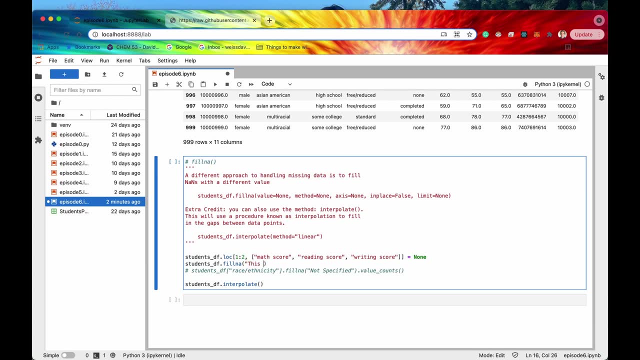 an l nna. what we can do is we can actually fill that value with another value, so we can actually add another value, cool. so what i'm going to do first here is say, i want to fill all of the missing values with this scalar, this string. right here, this value is missing and i also want to uh for these. 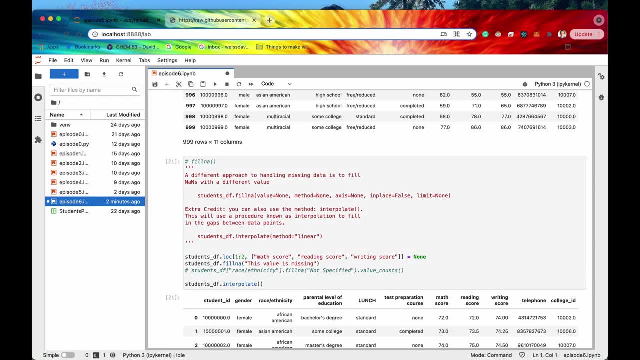 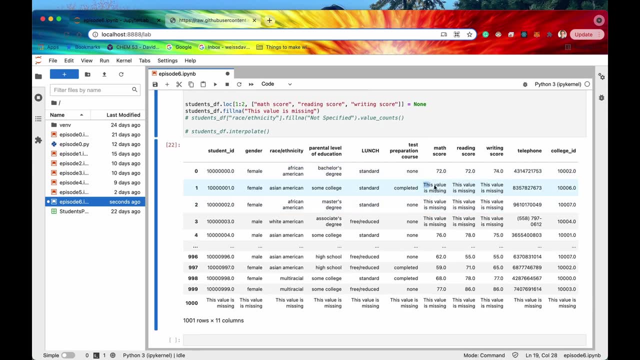 two rows. um, i'll also make those missing. awesome. so if i were to, oops- and i want to comment this out for now- awesome so, if i'm going to run this cell, then it looks like all of the nans, instead of the rows getting dropped, instead of the rows getting dropped, they actually got filled with. 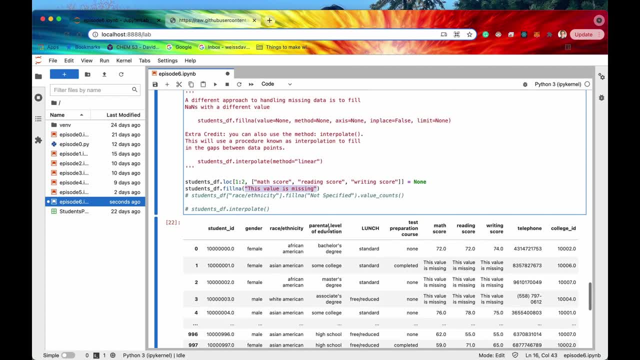 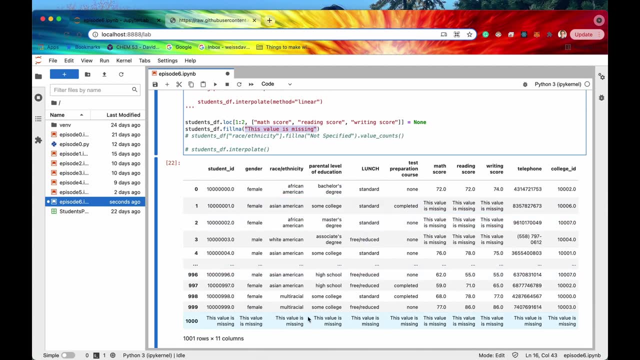 what we specified right here, cool. so this actually might not be the most ideal in every scenario because, again, if we were just to blanket fill every single uh value with, say, a string, this column right here, math score, you can see that all of these are floats, or at least they used to be. 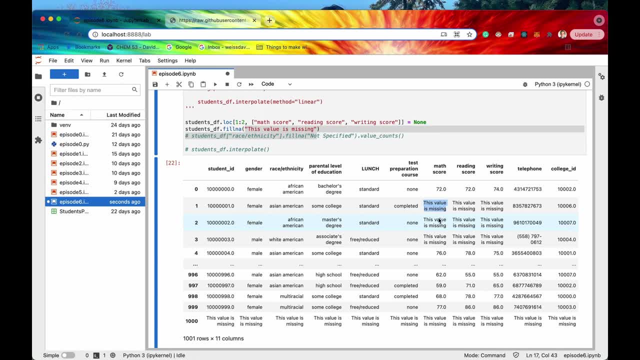 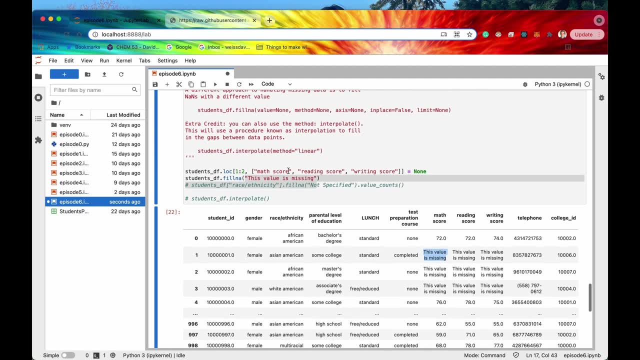 floats, right. so if we just specify it as a string, then that could mess up some data analysis, right? you can't really take that into account. so if we just specify it as a string, then that could make the average of 72 and this string right here. so maybe a better way of filling values is to use 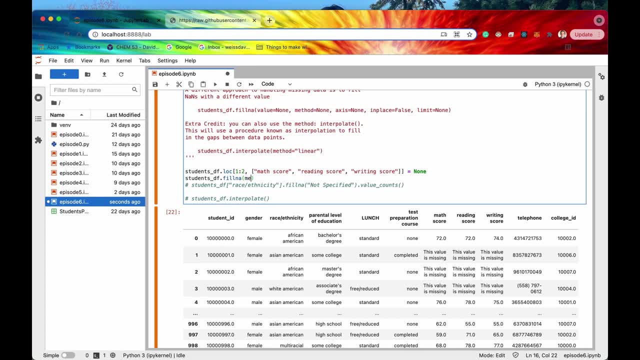 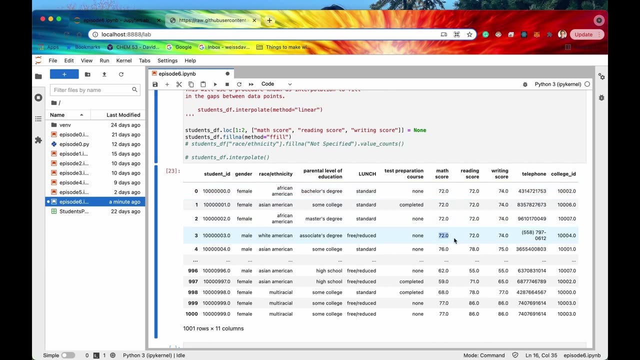 what's known as a method. so let's- uh, there are different methods that you can use, but let me demo one. let me demo first the forward fill method. cool, so this forward fill method. what this does is that when we encounter a missing value, then it's going to look backwards, it's going to look 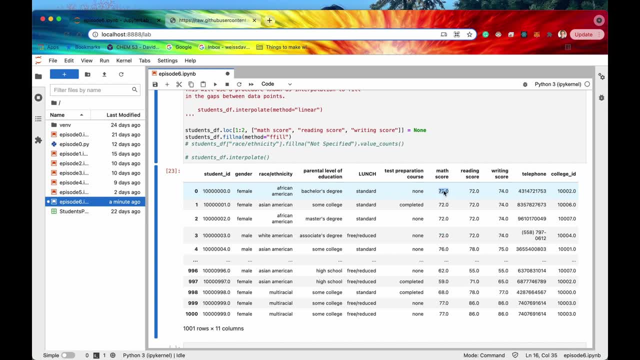 at the last uh non-missing value that we had and then just forward, fill that with uh throughout the rest of the missing values until we reach a non-missing value again. so again, if you recall, this used to be missing, this used to be missing, this used to be missing, uh. so what pandas did here is it took. 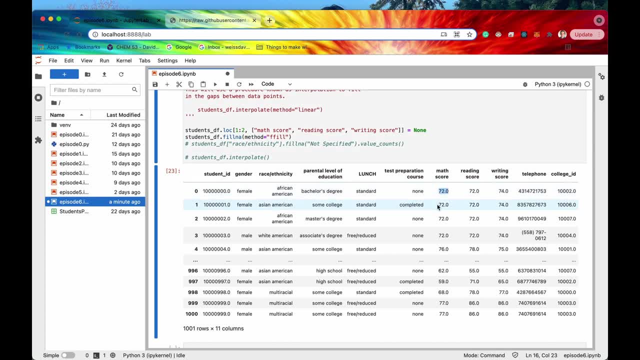 the last non-missing value and just copied that value into all of the or the, the following of values that are missing. so we've got 72, 72, 72, 72, and then we've got the non-missing value. now we have 76, because this again, this value was not missing. you can do a similar behavior by saying: 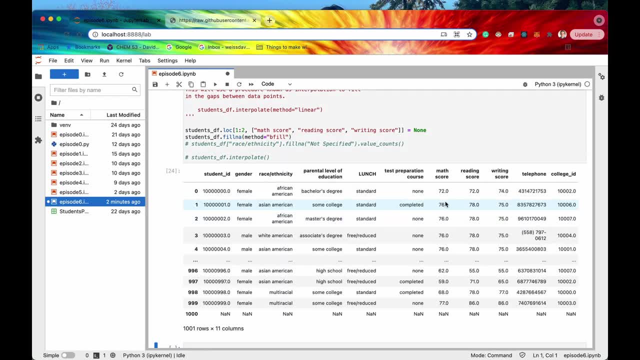 b fill, which stands for backfill, and what that does is that now, when we get missing values, we're just going to keep moving on until we get the next non-missing value and then we're going to backfill that, that that value that's not missing, into all of the missing values and just give it the same. 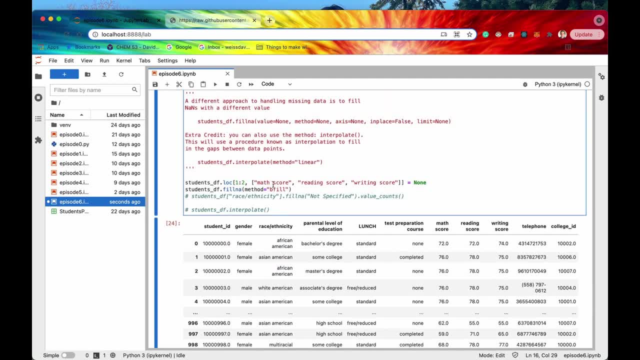 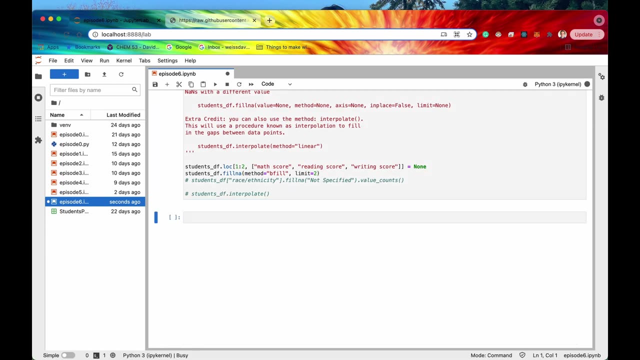 value. cool. so that is the backfill and forward fill methods. um, and then we also have like in place, we can specify a limit, and let me just show you what that does. so if i were to say limit equals one, then it's only going to backfill one time. if i were to say limit equals two, then that's going to say all right, you have a. 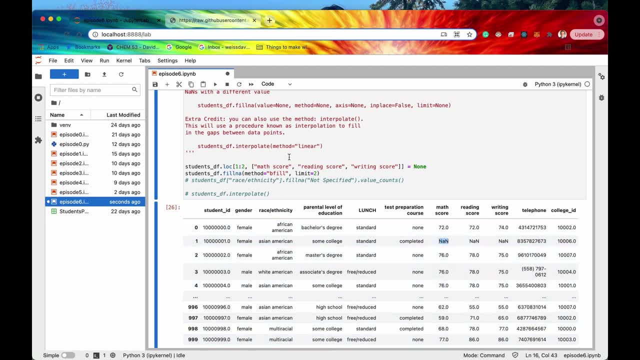 limit of two backfills but then after that stop backfilling. uh, and so this is just like a way to specify if you have like a limit for how many times you want to backfill or forward fill. um, that is how you can specify. cool, so fill in a can work on data frames. it can also work on. 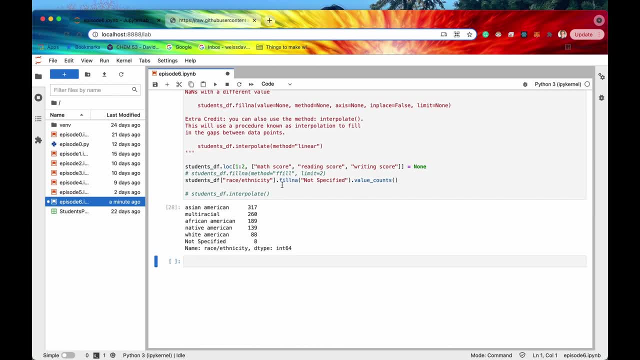 series itself. so if i were to run this here, we can see that we are filling in the series. any of the missing values in this column. we're going to just say not specified and, as you can see, there indeed we have eight values that have been filled with not specified. cool, so the last. 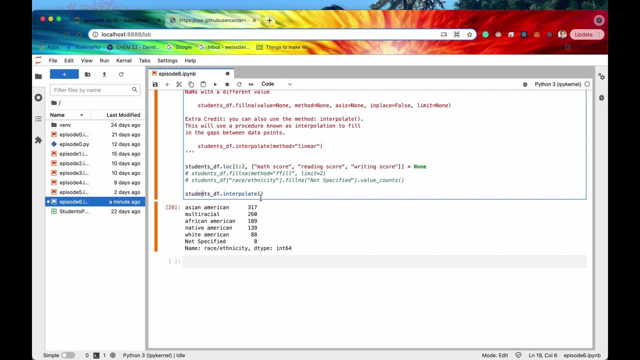 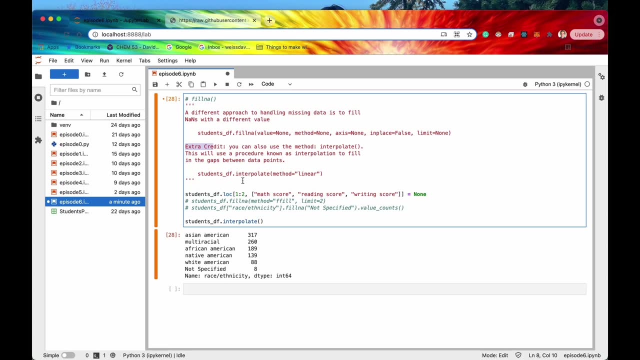 method that i want to look at before we wrap up. this video is interpolate, so i'm actually declaring this as extra credit. you don't technically need to know it. i don't use it that often, but it is a super cool method, so i decided to include it within. 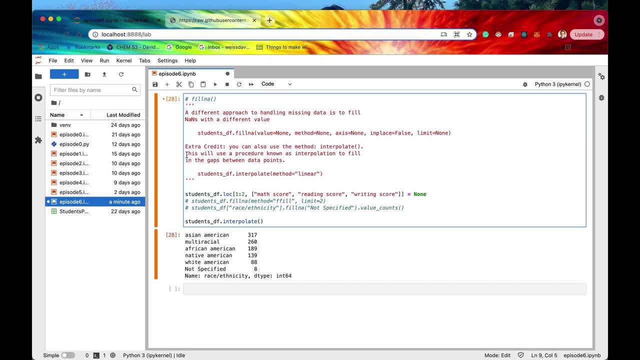 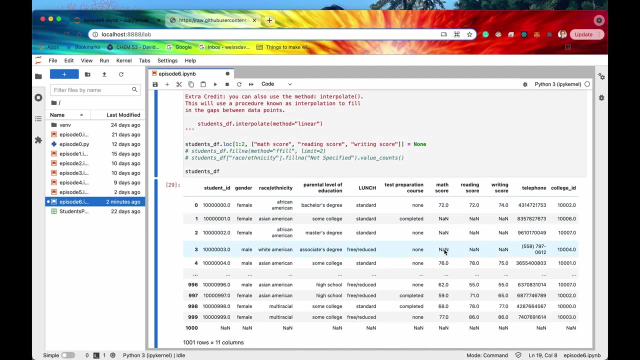 this method or this episode. so what interpolate will do is that it will run a procedure known as interpolation to fill the gaps in between data points. so, as a reminder, let me just show you what our data frame looks like right now. it has some missing values: n a n, n a n, n a n. 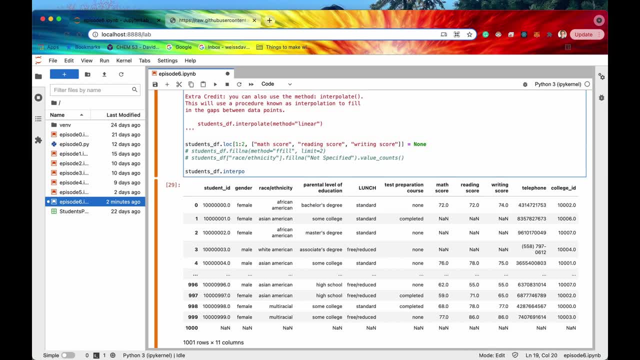 but if i were to fill in a can work on data frames, i would just say: fill in a can work on data frames were to run the interpolate method on it. watch what happens to these nans. so now, instead of just being like forward filled or back filled, what it does is it draws basically. 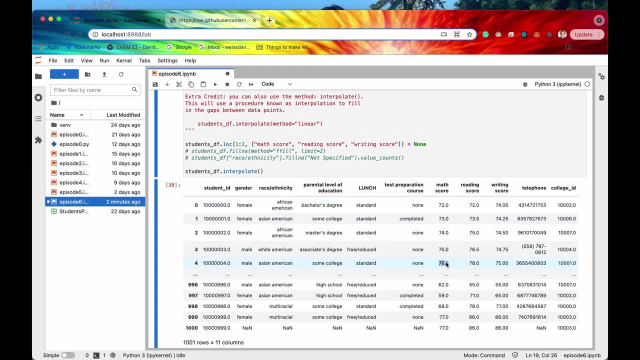 a line between 72 and 76 and it fills in all of the values, basically that attach 72 to 76 in a line. right, so it goes. now we are progressing. uh, one by one it goes 72, 73, 74, 75 and then 76. so